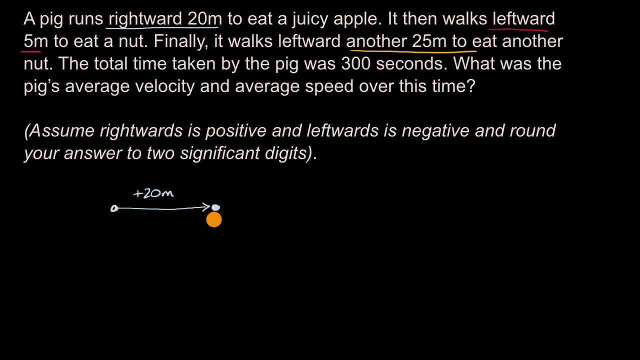 Then it walks leftwards five meters. So then from there it's going to walk leftwards five meters, So we could call that a negative five-meter displacement. And then finally it walks leftward another 25 meters. So then it walks leftward another 25 meters. 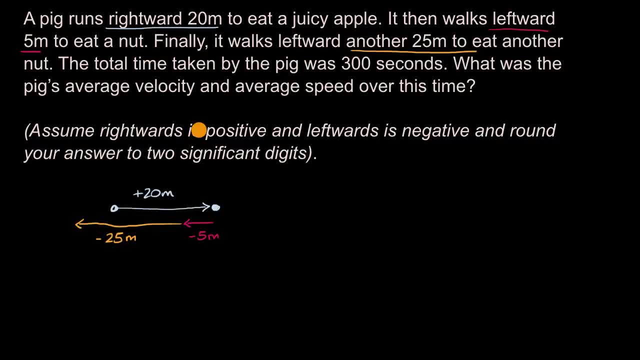 So it gets right over there. So that'd be a displacement of negative 25 meters to eat another nut. So it ends up right over. it ends up right over there. Now to figure out our average velocity, let me write it down. 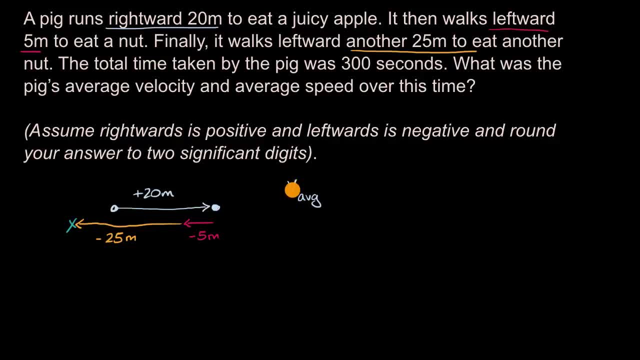 So our velocity average, And even though this is one-dimensional, it is a vector. It has direction to it. We specify the direction with the sign rightwards being positive and leftwards being negative. You oftentimes for one-dimensional vectors. 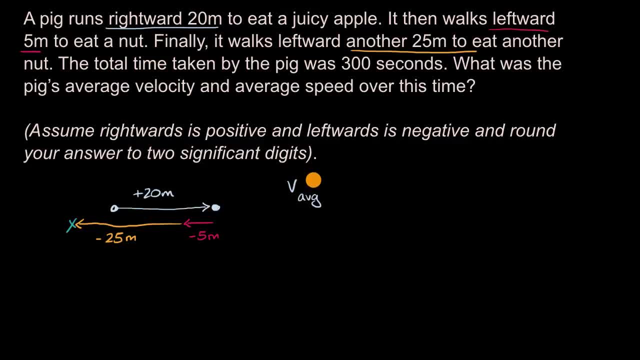 might not see an arrow there or might not see it bolded and just written like this, But our average velocity is going to be equal to. you could view it as our displacement, or a change in x divided by how much time has actually left. 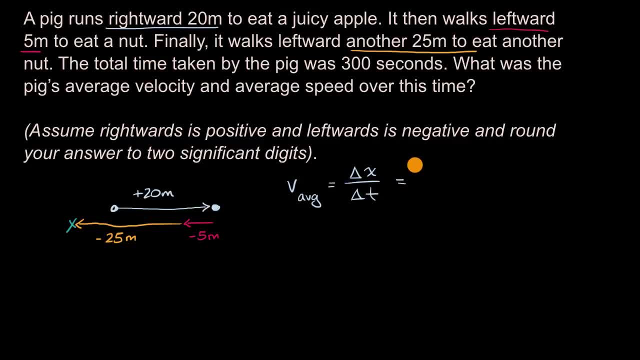 It's going to be the time that the velocity has elapsed, And so what is our displacement going to be? Let's see, we have plus 20 meters, And then we have minus five meters, And then we go to the left another 25 meters. 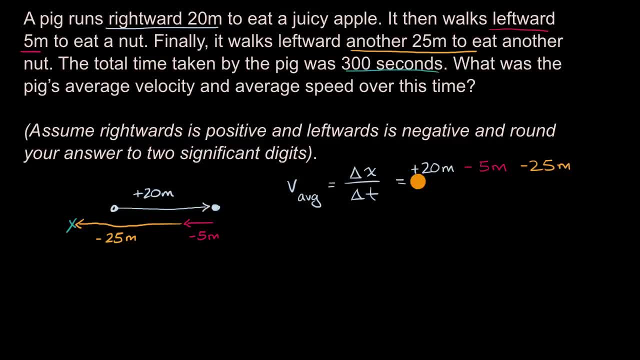 Minus 25 meters, And then all of that is going to be over the elapsed time or change in time. All of that is over 300 seconds. So what is this numerator going to be? This is 20 minus 30.. 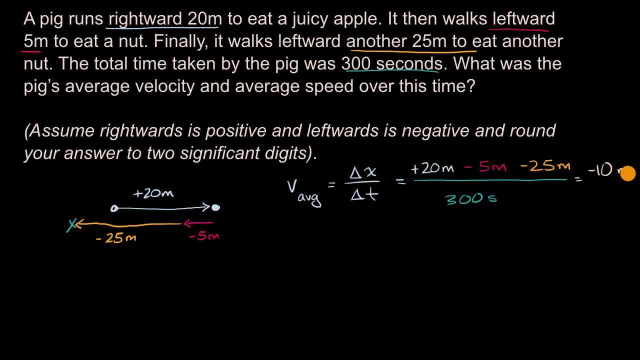 So that's going to be equal to negative 10.. So that's going to be equal to negative 10 meters over 300 seconds, over 300 seconds. So the average velocity is going to be equal to negative 1 30th meters per second. 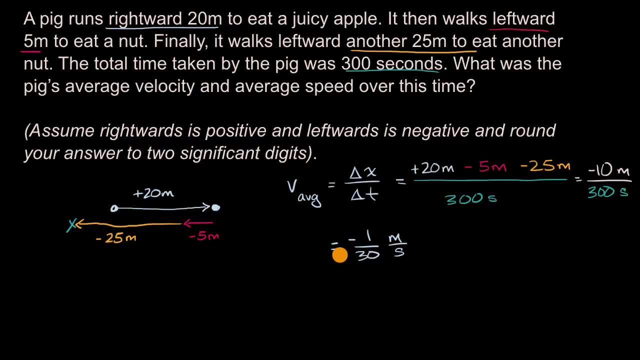 The negative specifies that, on average, the velocity is towards the left. If you want to specify this as a decimal with two significant digits, this is going to be so. it's approximately equal to 0.05.. 0.033, that would be 1, 30th. 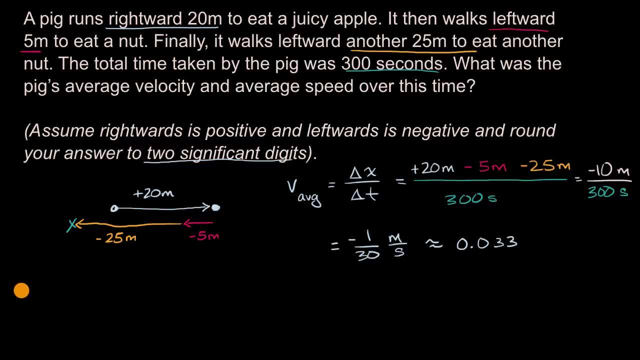 Now let's try to tackle average speed. So our speed r sometimes is used for speed, r, for rate. Our average speed is not going to be our displacement divided by our elapsed time. It is going to be our distance divided by our elapsed time. 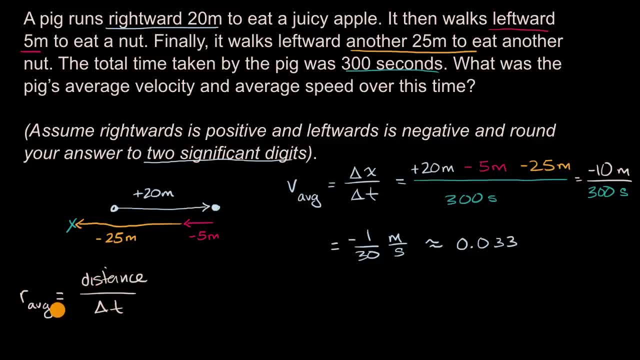 And we'll see that these are not going to be the same thing. That's one of the points of this problem. So, our distance divided by elapsed time, Our distance traveled, What's going to be the absolute value of each of these numbers? 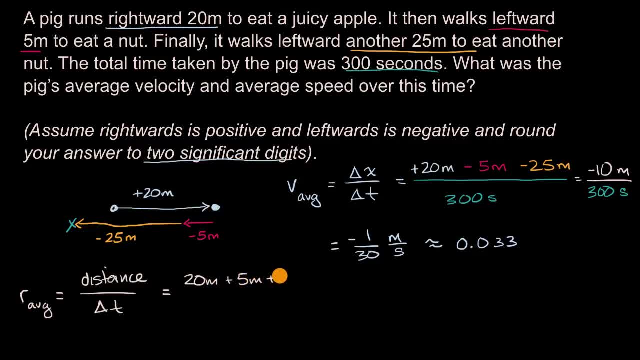 So it's going to be 20 meters plus five meters plus 25 meters. Notice there's a difference here. We're not subtracting the five and the 25. We're just adding all of that. We just care about the magnitudes. 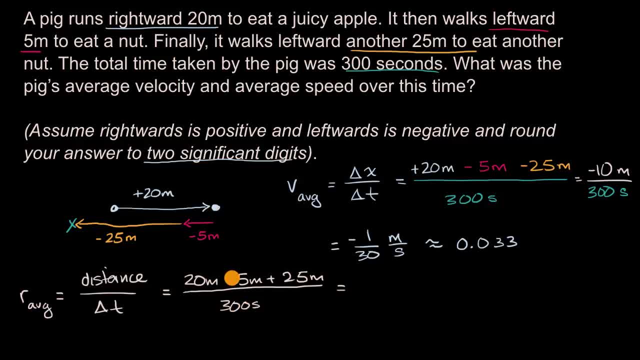 Divided by 300 seconds, And so this is going to be equal to 50 meters. 50 meters over 300 seconds, which is equal to five over 30, which is equal to 1: 30th, That's 1, 6th of a meter per second. 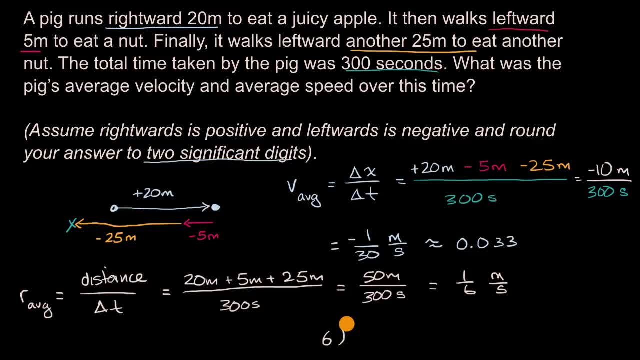 And if we want to write it as a decimal, let's see: six goes into one. Let's put some zeros here: Six goes into 10.. One time, one times six is six. I could scroll down a little bit, And then we subtract. 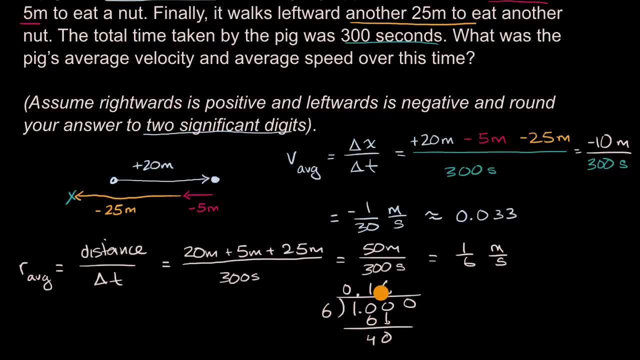 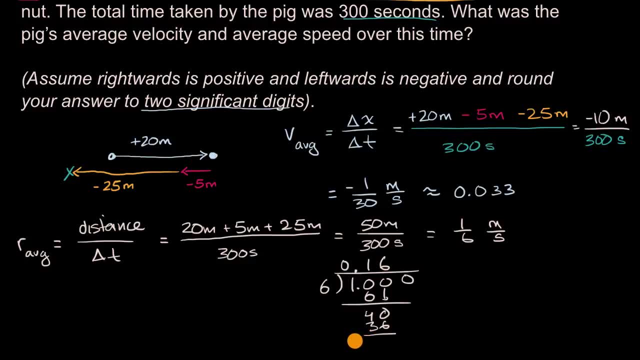 We get a four. Six goes into 40, six times Six times six is 36.. And we're still. and then we get- let me scroll down a little bit more again- And then we get another six, We get another, we get another four. 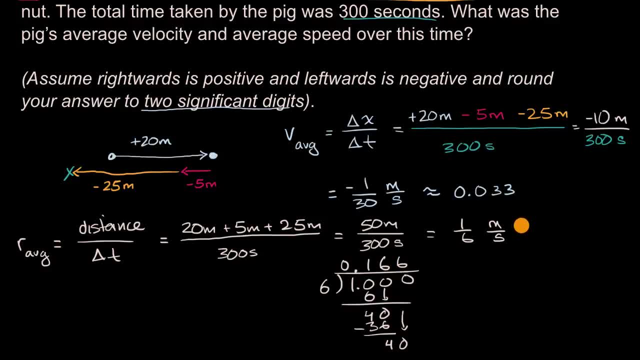 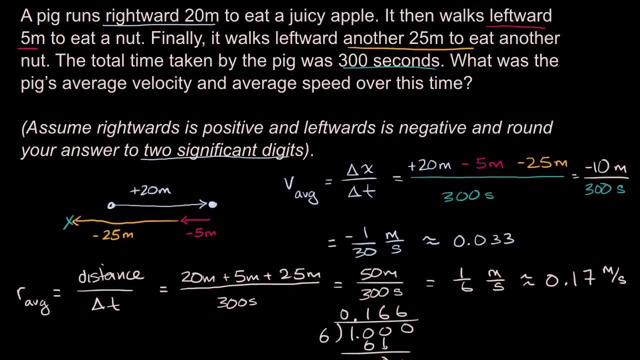 And then we're just gonna keep getting sixes over here. So this is going to be approximately equal to 0.1,. if we want two significant digits, one, seven meters per second, And we are done. We figured out the average velocity and the average speed.